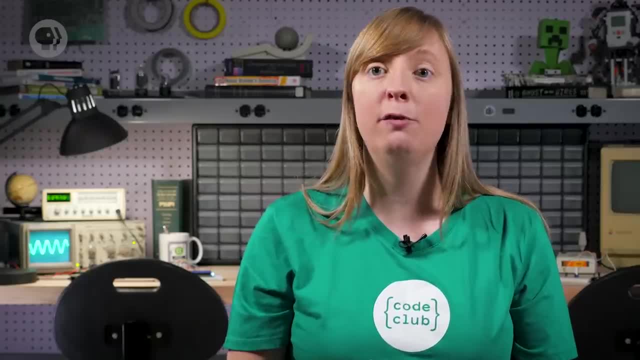 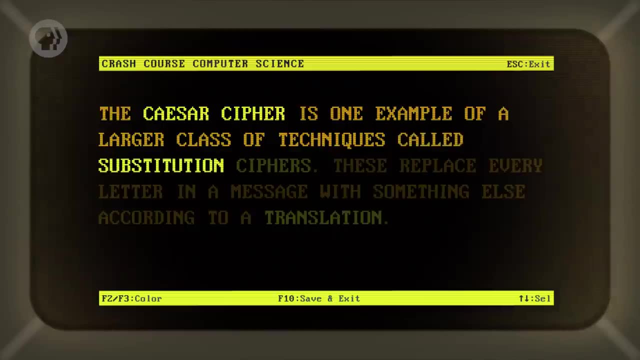 Brutus became this. To decipher the message, recipients had to know both the algorithm and the number to shift, by which acted as the key. The Caesar cipher is one example of a larger class of techniques called substitution ciphers. These replace every letter in a message with something else according to a translation. 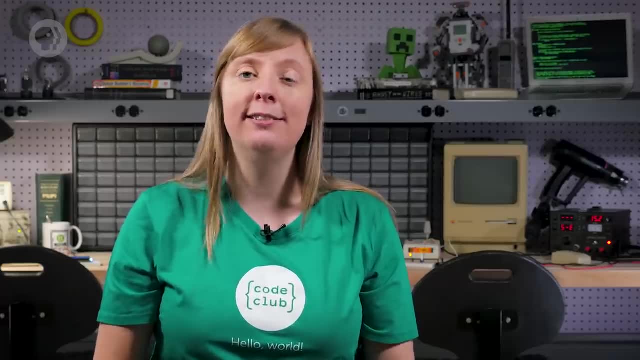 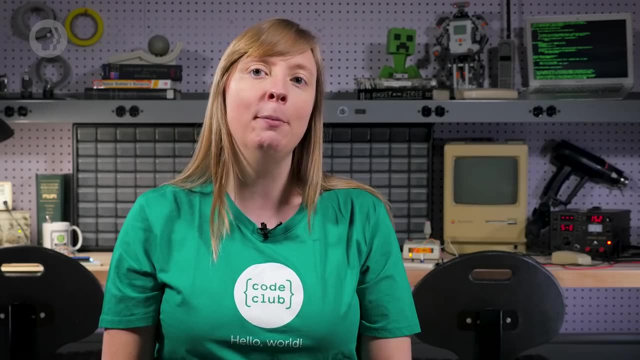 A big drawback of basic substitution ciphers is that letter frequencies are preserved. For example, E is the most common letter in English, So if your cipher translates E to an X, then X will show up the most frequently in the ciphertext. A skilled cryptanalyst can work backwards from these kinds of statistics to figure out. 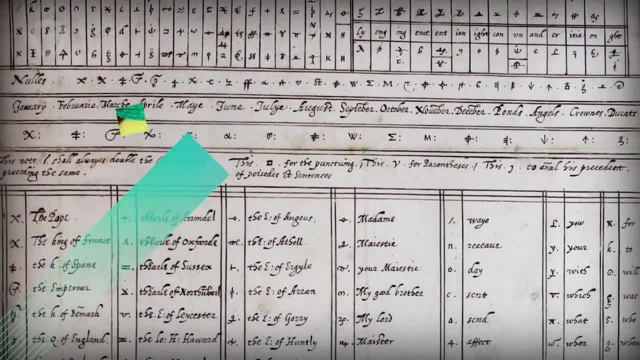 the message. It was the breaking of a substitution cipher that led to the execution of Mary, Queen of Scots, which is a very common letter in English. It's a very common letter in English and it was used in 1587 for plotting to kill Queen Elizabeth. 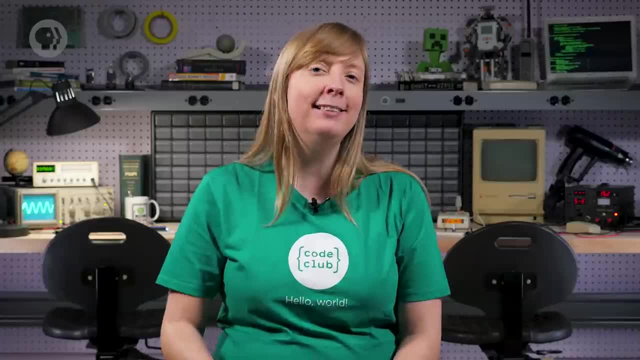 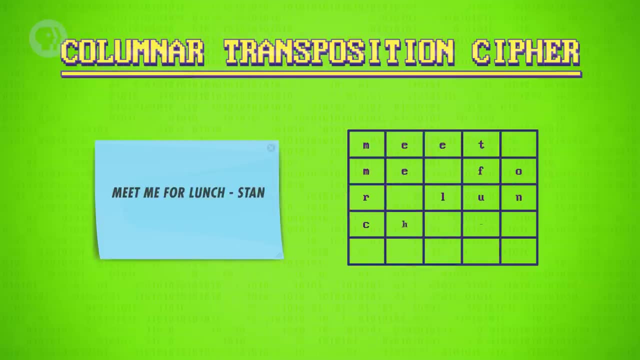 Another fundamental class of techniques are permutation ciphers. Let's look at a simple example called a commonar transposition cipher. Here we take a message and fill the letters into a grid. In this case, we've chosen 5 by 5.. 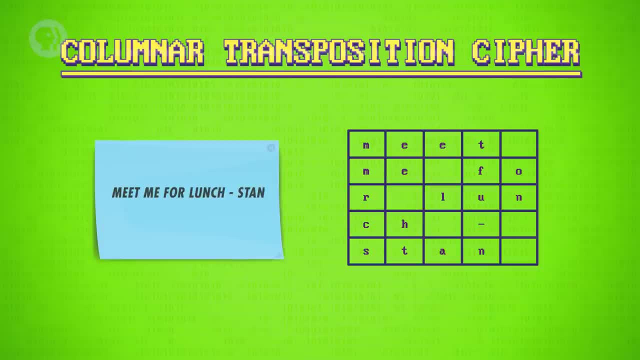 To encrypt our message, we read out the characters in a different order, Let's say from the bottom left, working upwards, one column at a time. The new letter ordering what's called a permutation is the encrypted message, The ordering direction, as well as the 5 by 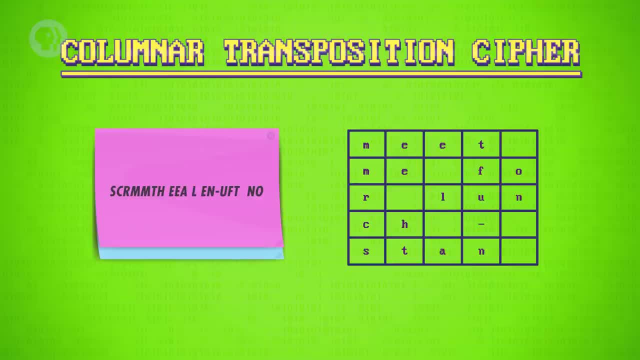 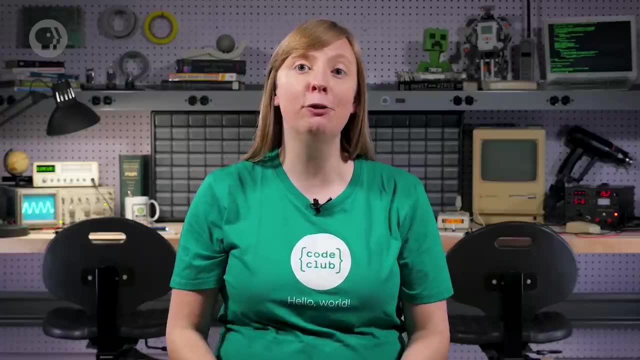 5. grid size serves as the key. Like before, if the cipher and key are known, a recipient can reverse the process to reveal the original message. By the 1900s, cryptography was mechanized in the form of encryption machines. The most 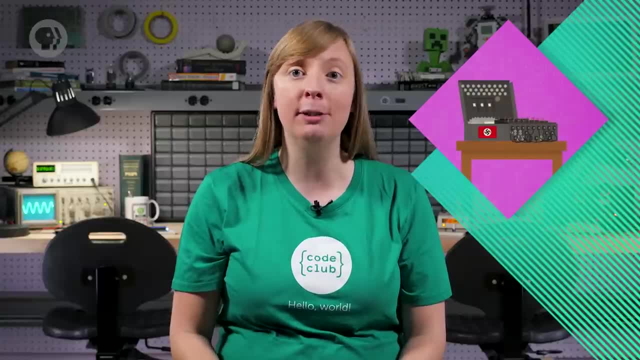 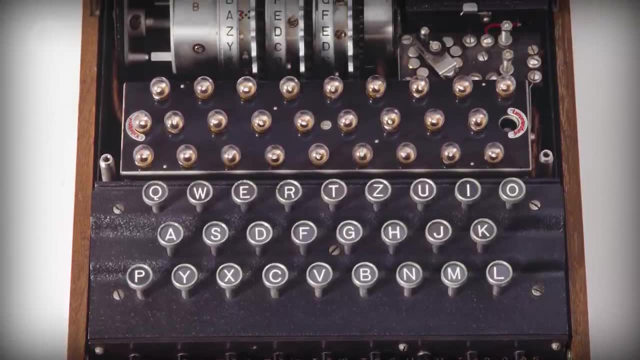 famous was the German Enigma, used by the Nazis to encrypt their wartime communications. As we discussed back in episode 15,, the Enigma was a typewriter-like machine with a keyboard and lamp board, both showing the full alphabet. Above that there was a series of configurable. 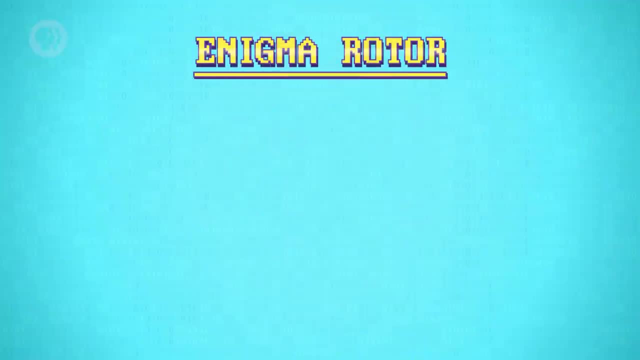 rotors that were the key to the Enigma's encryption capability. First let's look at just one rotor. One side had electrical contacts for all 26 letters. These connected to the other side of the rotor using cross-crossing wires that swapped one letter for another. 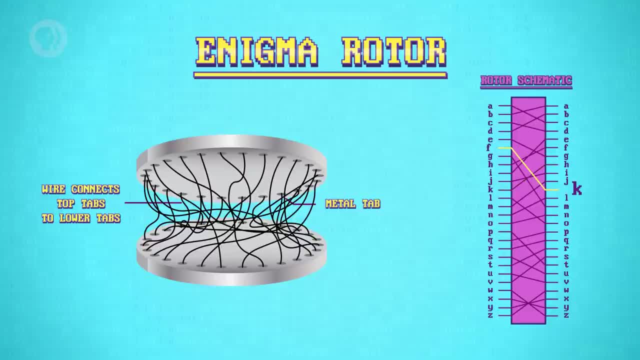 If H went in, K might come out. the other side, If K went in, F might come out, and so on. The letter-swapping behavior should sound familiar. It's a substitution cipher, but the Enigma was more sophisticated because it used three or more rotors in a row each. 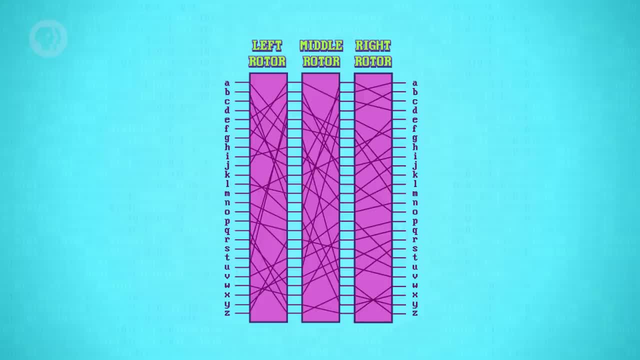 feeding into the next Rotors could also be rotated to one of 26 possible starting positions And they could be inserted in different orders, providing a lot of different substitution mappings. Following the rotors was a special circuit called a reflector, Instead of passing. 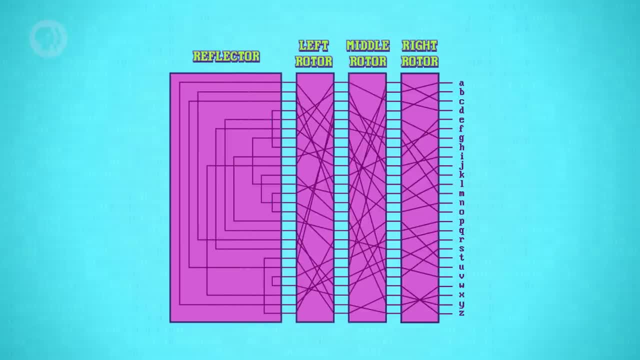 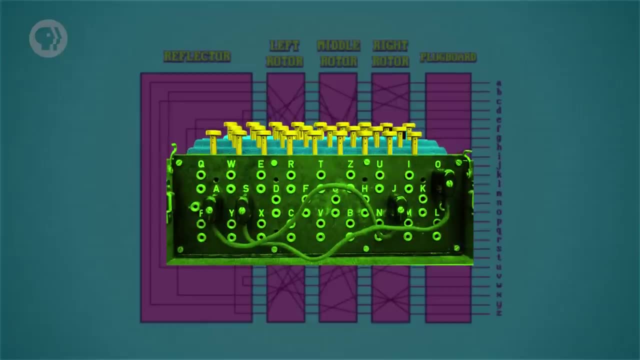 the signal onto another rotor. it connected every pin to another and sent the electrical signal back through the rotors. Finally, there was a plug board at the front of the machine that allowed letters coming from the keyboard to be optionally swapped, adding another level. 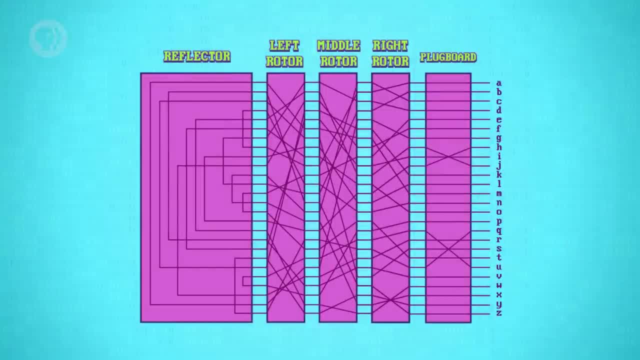 of complexity With our simplified circuit. let's encrypt a letter on this example: Enigma configuration. If we press the H key, electricity flows through the rotors, hits the reflector, comes back through the rotors and plug board and illuminates. 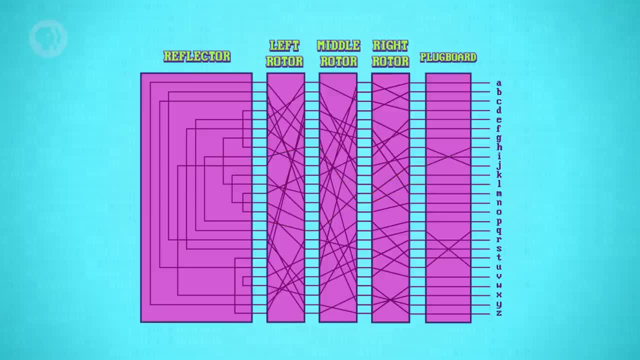 the letter L on the lamp board. So H is encrypted to L. Note that the circuit can flow both ways. So if we type the letter L, H would light up. In other words, it's the same process for encrypting and decrypting. You just have. 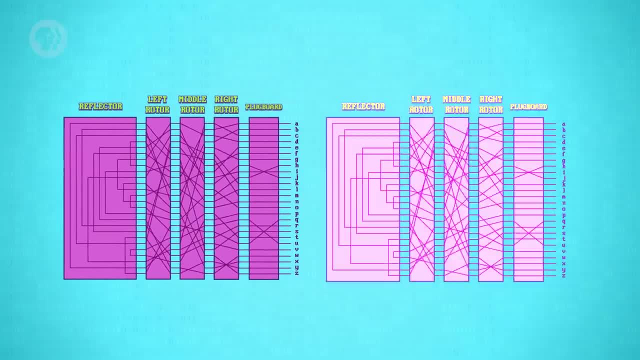 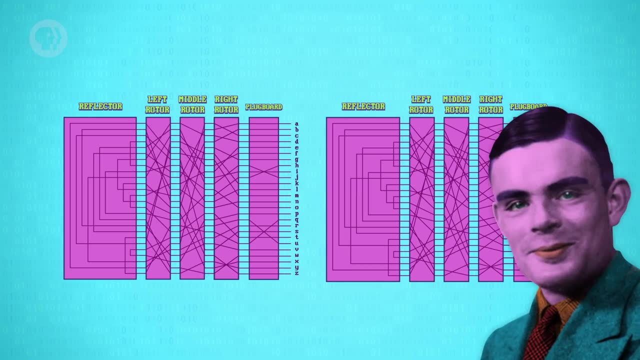 to make sure the sending and receiving machines have the same initial configuration. If you look carefully at this circuit, you'll notice it's impossible for a letter to be encrypted as itself, which turned out to be a fatal cryptographic weakness. Finally, to prevent the Enigma from being a simple circuit, we'll use the Enigma to 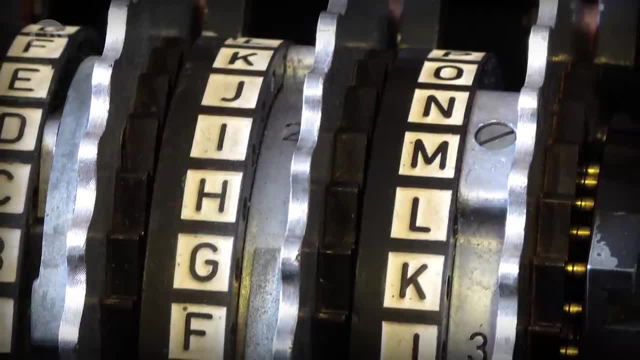 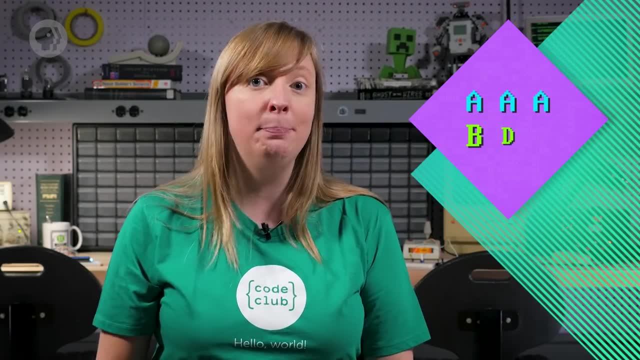 be a simple substitution cipher. Every single time a letter was entered, the rotors advanced by one spot, sort of like an odometer in a car. So if you entered the text AAA, it might come out as BDK, where the substitution mapping changed with every key press. 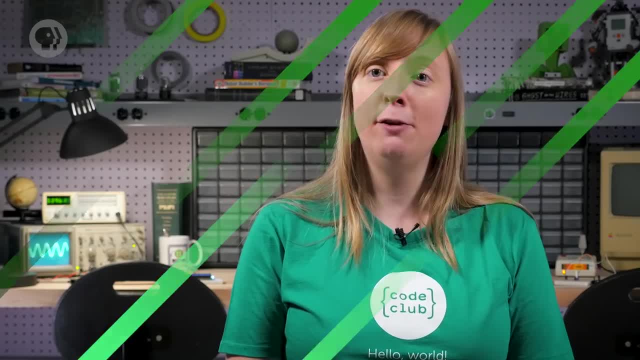 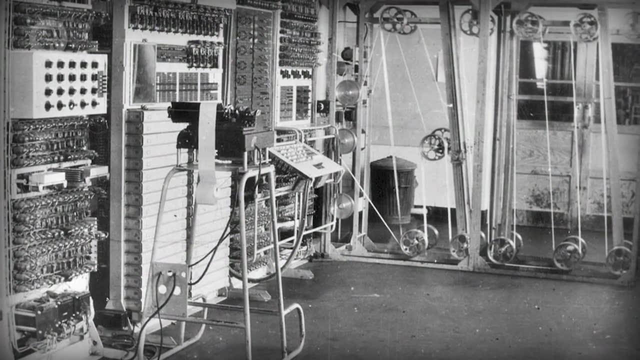 The Enigma was a tough cookie to crack, for sure, but, as we discussed in episode 15,, Alan Turing and his colleagues at Bletchley Park were able to break Enigma codes and largely automate the process. But with the advent of computers, cryptography, 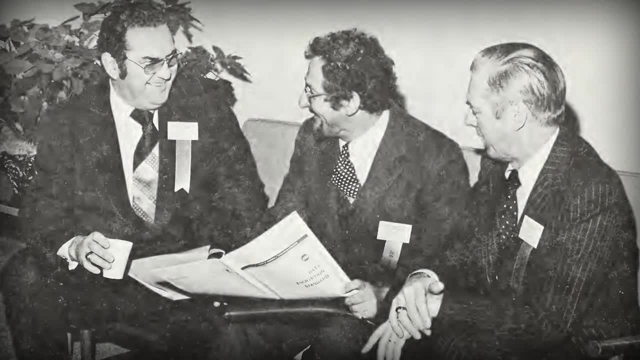 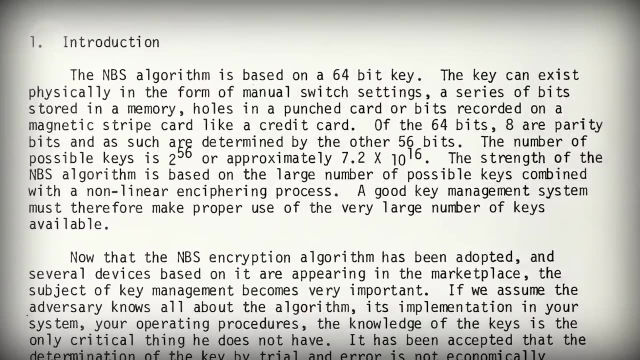 moved from hardware into software. One of the earliest software ciphers to become widespread was the Data Encryption Standard developed by IBM and the NSA in 1977.. DES, as it was known, originally used binary keys that were 56 bits long, which means that there. 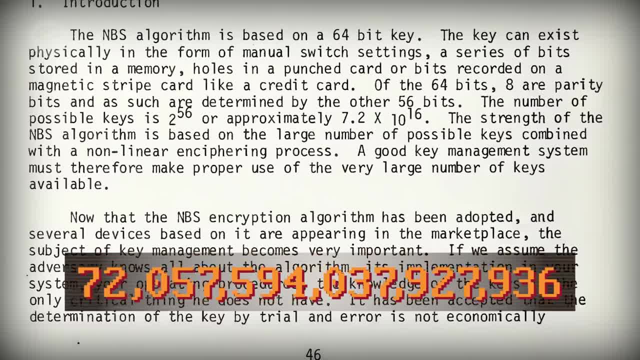 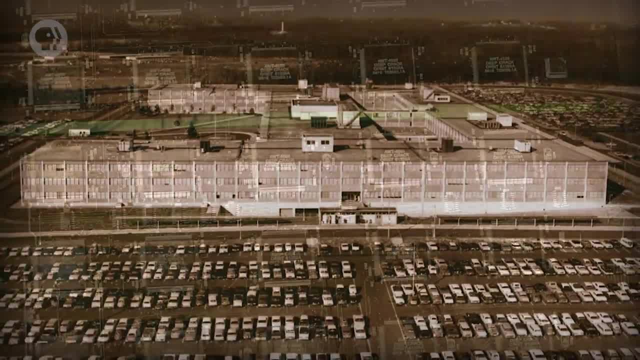 are 2 to the 56, or about 72 quadrillion different keys. Back in 1977, that meant that nobody, except perhaps the NSA, had enough computing power to brute force all possible keys. But by 1999, a quarter million dollar computer could try. 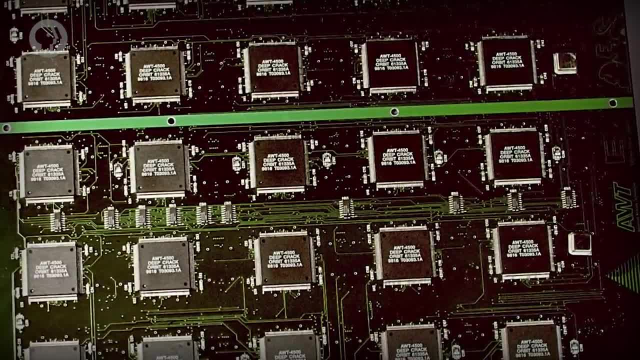 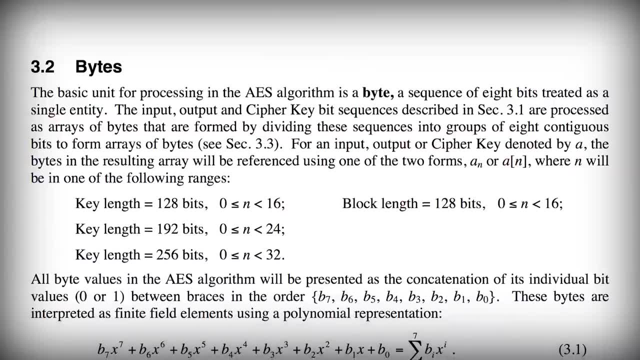 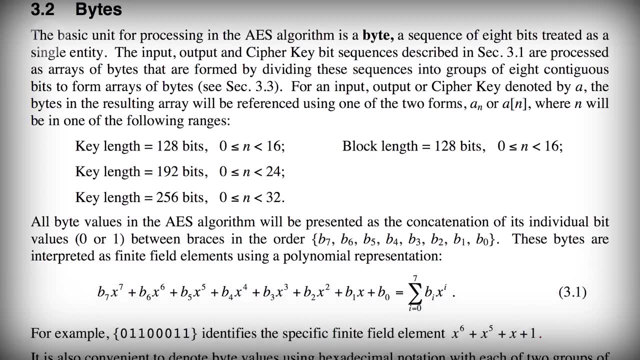 every possible DES key in just two days, rendering the cipher insecure. So in 2001,, the Advanced Encryption Standard, AES, was finalized and published. AES is designed to use much bigger keys: 128,, 192, or 256 bits in size, making brute force attacks much. 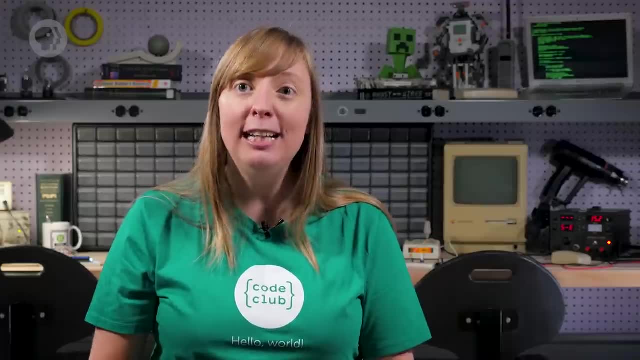 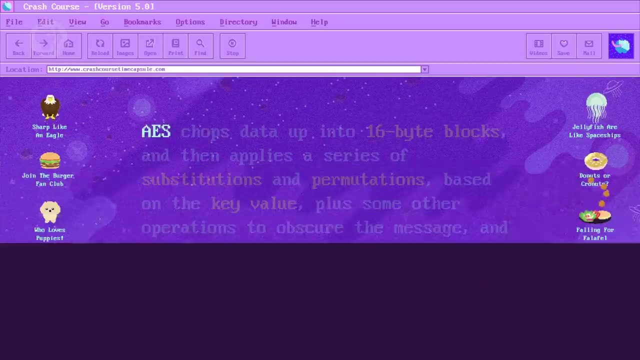 much harder. For a 128-bit key. you'd need trillions of years to try every combination, even if you used every single computer on the planet today, So you'd better get started. AES chops data up into 16-byte blocks and then applies a series of substitutions and 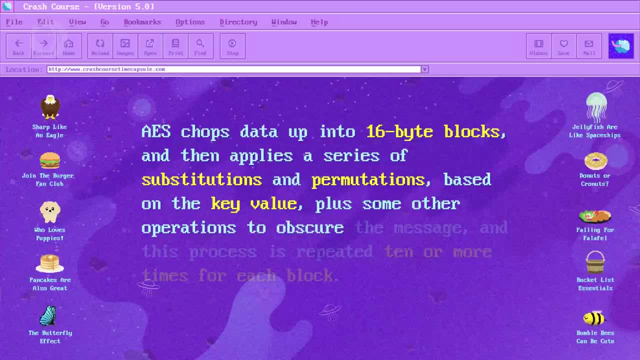 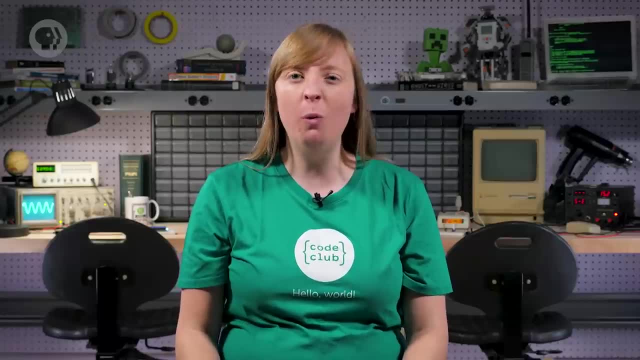 permutations based on the key value, plus some other operations to obscure the message, And this process is repeated 10 or more times for each block. You might be wondering why only 10 rounds, Or why only 128-bit keys and not 10,000-bit. keys. Well, it's a performance trade-off. If it took hours to encrypt and send an email, or minutes to connect to a secure website, people wouldn't use it. AES balances performance and security to provide practical cryptography. Today, AES is used. 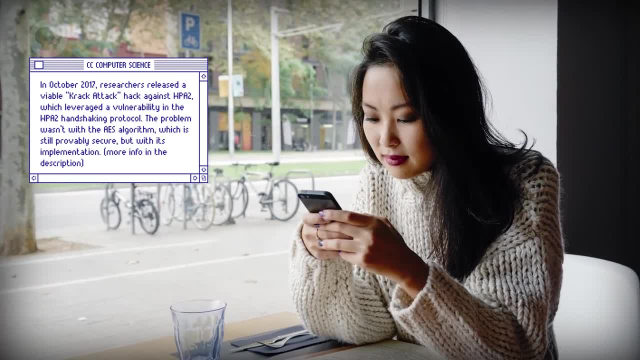 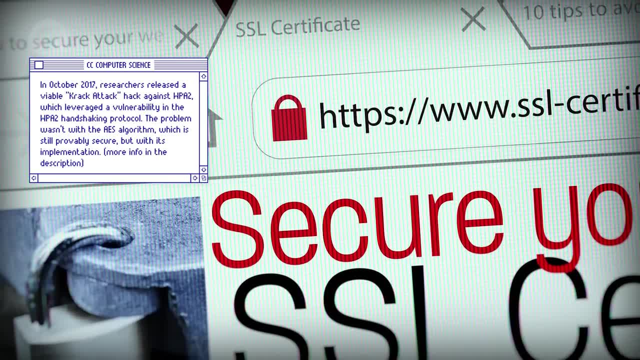 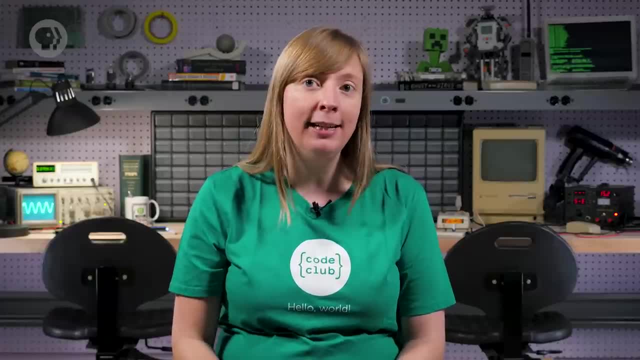 It's been used for a long time. It's been used for a long time So far. the cryptographic techniques we've discussed rely on keys that are known by both sender and recipient. The sender encrypts a message using a key and the recipient decrypts. 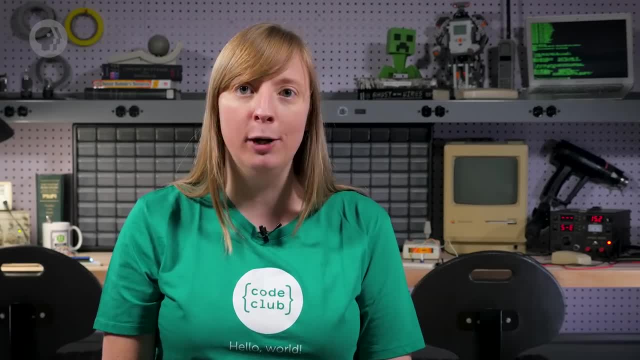 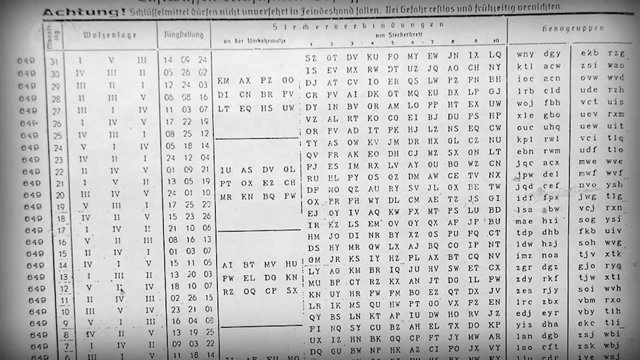 it using the same key. In the old days, keys would be shared by voice or physically. For example, the Germans distributed code books with daily settings for their Enigma machines, But this strategy could never work in the internet era. Imagine having to crack open a code book to connect to YouTube. 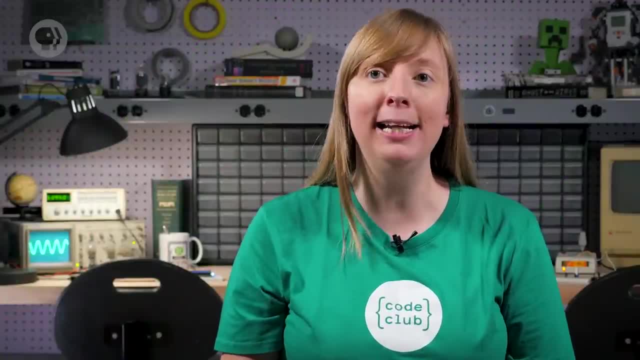 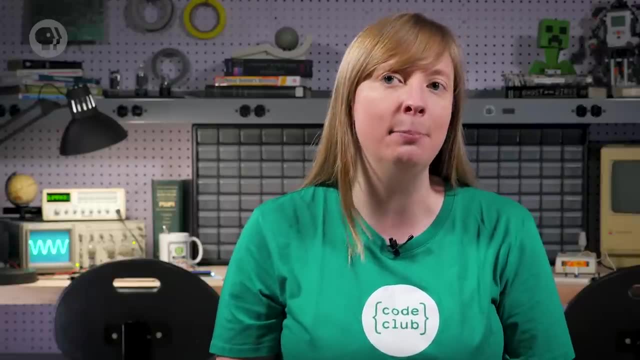 What's needed is a way for a server to send a secret key over the public internet to a user wishing to connect securely. It seems like that wouldn't be secure, because if the key is sent in the open and intercepted by a hacker, couldn't they use that to decrypt all communication between the two? 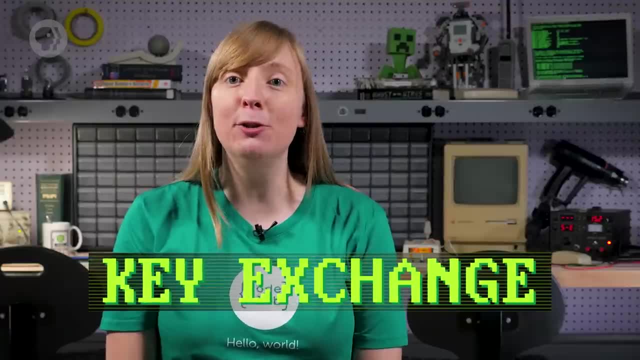 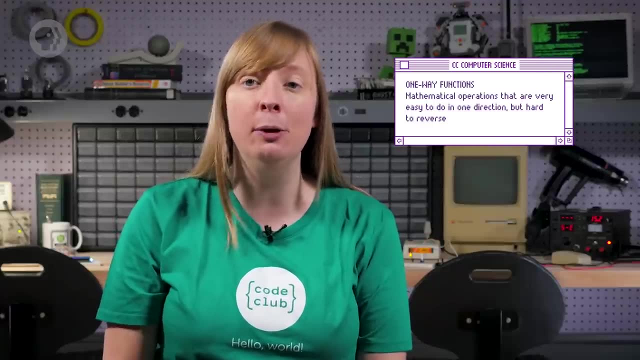 The solution is key exchange, an algorithm that lets two computers agree on a key without ever sending one. We can do this with one-way functions, mathematical operations that are very easy to do in one direction but hard to reverse. To show you how one-way functions work, let's use paint colors as an analogy. 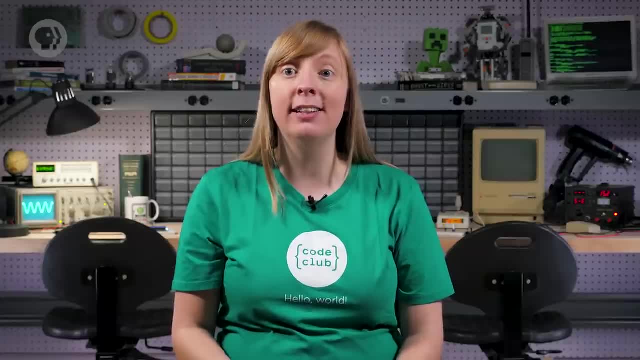 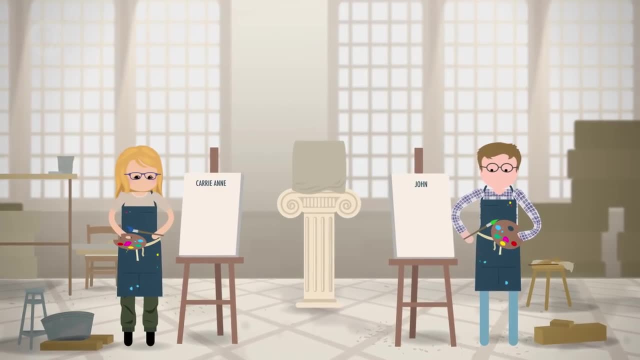 It's easy to mix paint colors together, but it's not so easy to figure out the constituent colors that we use to make a mixed paint color. You'd have to test a lot of possibilities to figure it out. In this metaphor, our secret key is a unique shade of paint. 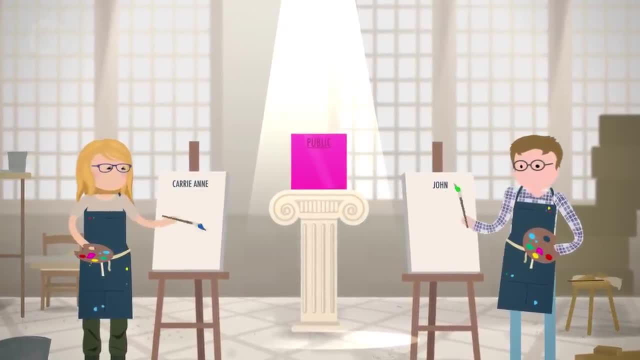 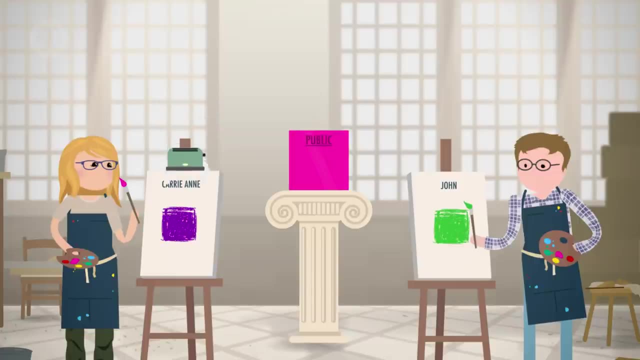 First there's a public paint color that everyone can see. Then John and I each pick a secret paint color To exchange keys. I mix my secret paint color with the public paint color. Then I send that mixed color to John. by any means. 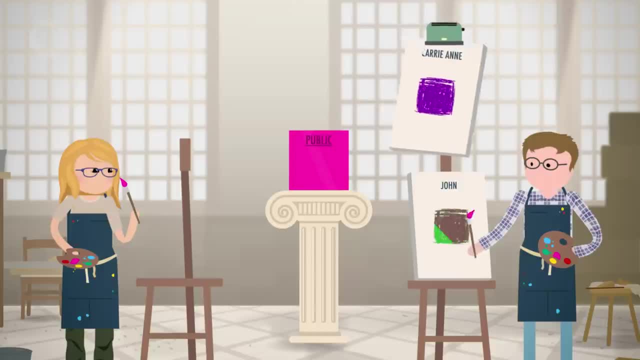 Male, Female, Male, ich mean whatever. John does the same, mixing his secret paint color with the public color, then sending that to me. When I receive John's color, I simply add my private color to create a blend of all three paints. 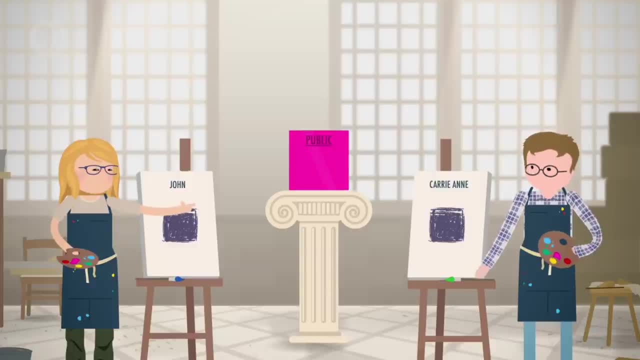 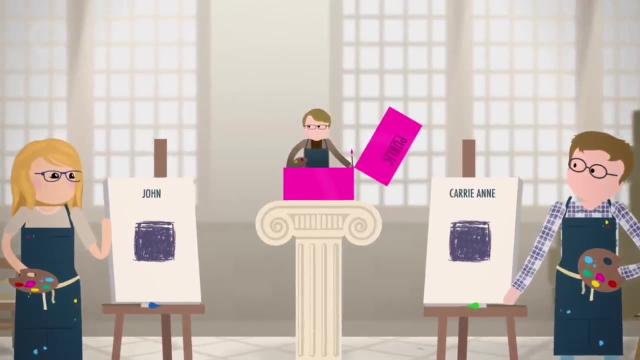 John does the same with my mixed color and voila, We both end up with the same paint color. We can use this as a shared secret, even though we never sent each other our individual secret colors. A snooping outside observer would know partial information, but they'd find it very difficult. 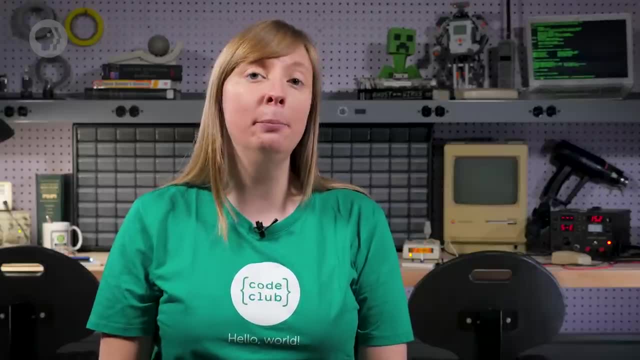 to figure out our shared secret color. Of course, sending and mixing paint colors isn't going to work well, for 좋과겠습니다 transmitting computer data, But luckily mathematical one-way functions are perfect, and this is what Diffie-Hellman. 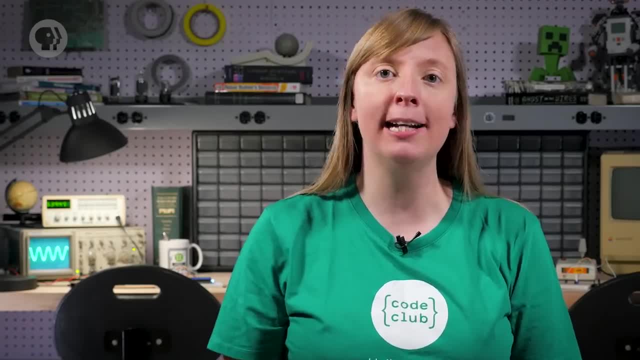 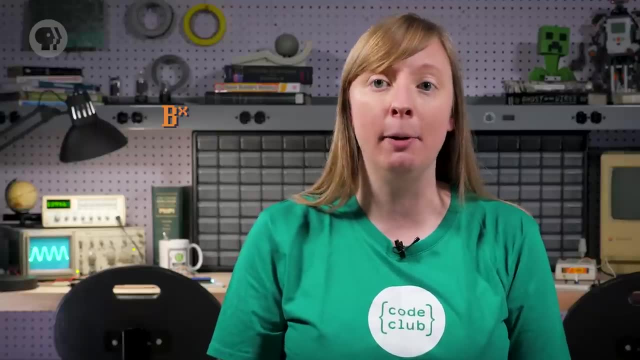 Key Exchange uses. In Diffie-Hellman, the one-way function is modular exponentiation. This means taking one number, the base, to the power of another number, the exponent, and taking the remainder when divided by a third number, the modulus. 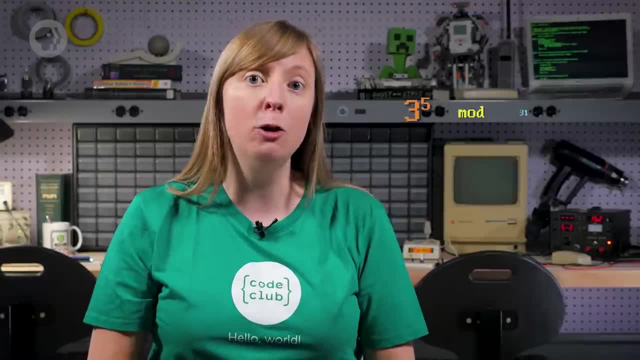 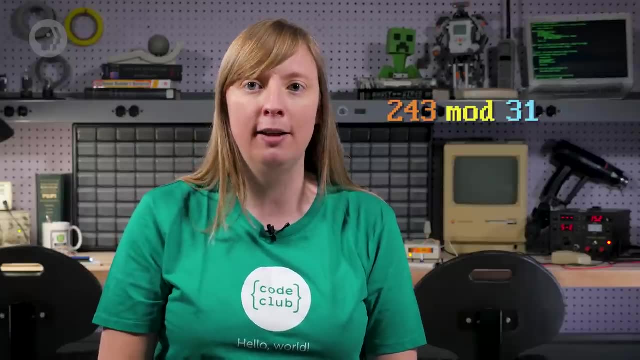 So, for example, if we wanted to calculate three to the fifth, power modulo thirty-one, we would calculate three to the fifth, which is two hundred and forty-three, and then take the remainder when divided by thirty-one, which is twenty-six. 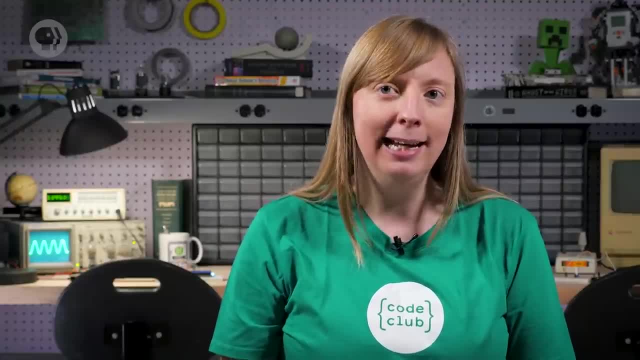 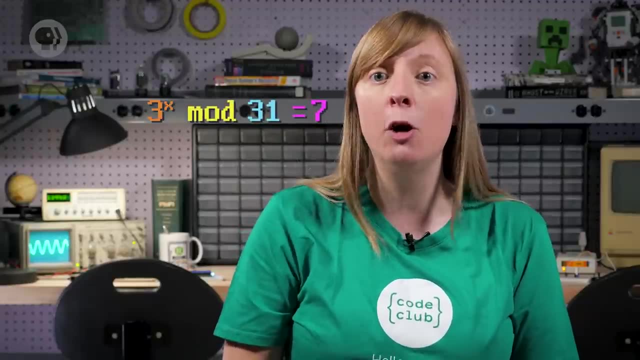 The hard part is figuring out the exponent, given only the result and the base. If I tell you, I raised three to some secret number modulo thirty-one and got seven as the remainder. you'd have to test a lot of exponents to know which one I picked. 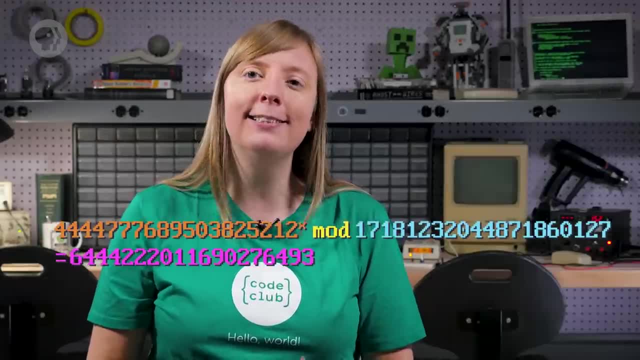 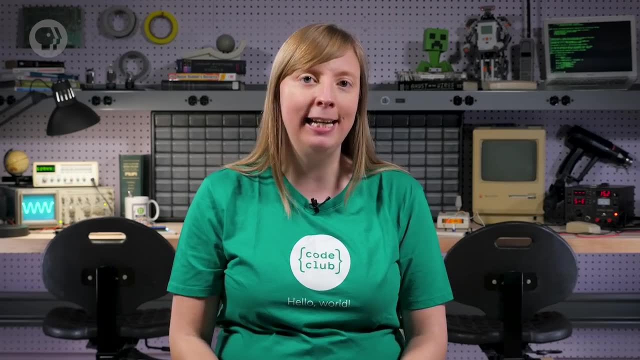 If we make these numbers big, say hundreds of digits long, then finding the secret exponent is nearly impossible. Now let's talk about how Diffie-Hellman uses modular exponentiation to calculate a shared key. First there's a set of public values: the base and the modulus. 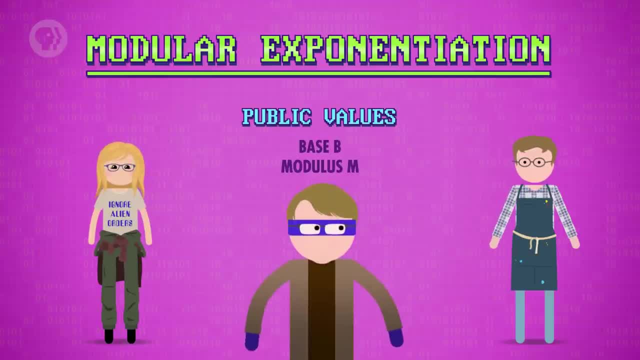 But like our public paint color, everyone gets to know, Even the bad guys. To send a message securely to John, I would pick a secret exponent, x, then I'd calculate b to the power of x modulo m. I send this big number over to John. 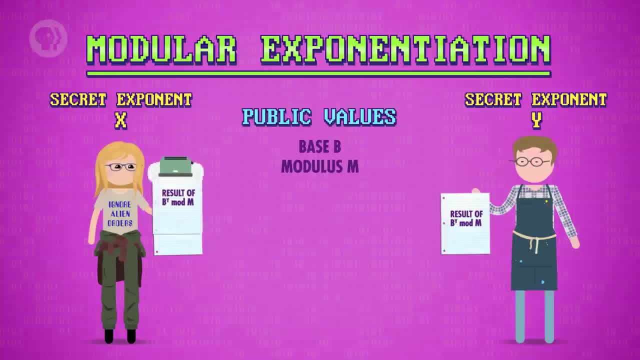 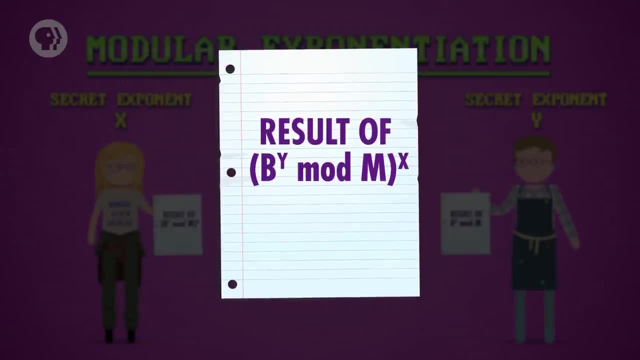 John does the same, picking a secret exponent, y, and sending me b to the y modulo m To create a shared secret key. I take what John sent me and take it to the power of x, my secret exponent. This is mathematically equivalent to b to the xy modulus m. 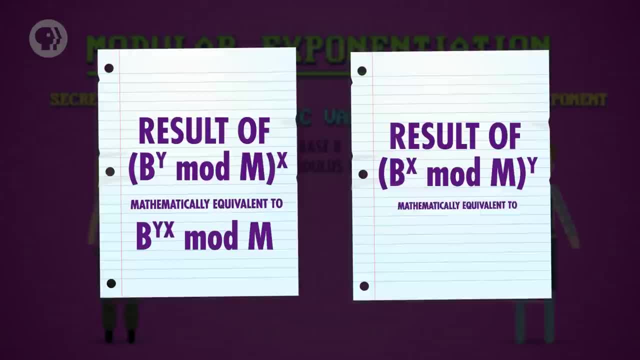 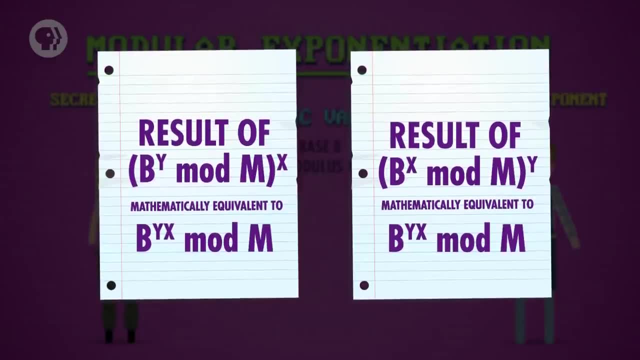 John does the same. I'm taking what I sent to him to the power of y and we both end up with the exact same number. It's a secret shared key. even though we never sent each other our secret number, We can use this big number as a shared key for encrypted communication using something. 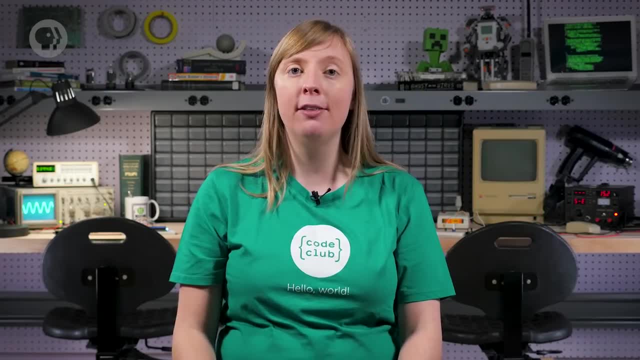 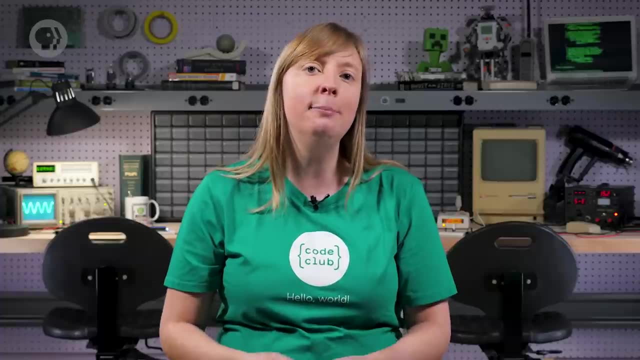 like AES for encryption, Diffie-Hellman key exchange is one method for establishing a shared key. These keys that can be used by both sender and receiver to encrypt and decrypt messages are called symmetric keys, because the key is the same on both sides. 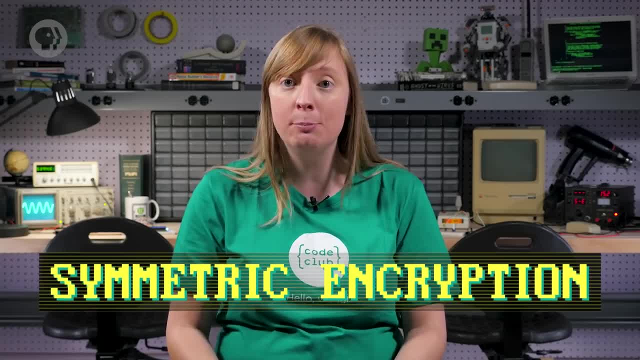 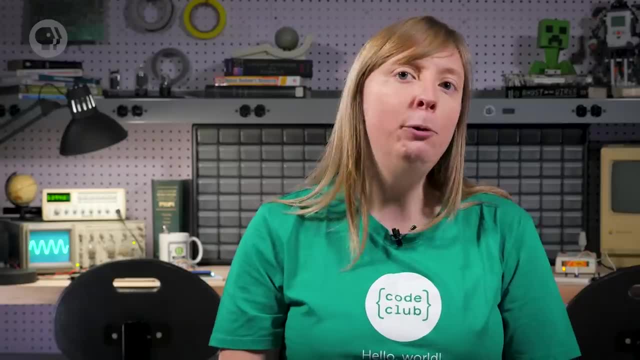 The Caesar cipher enigma and AES are the same. There's also asymmetric encryption, where there are two different keys, most often one that's public and another that's private. So people can encrypt a message using a public key that only the recipient with their private. 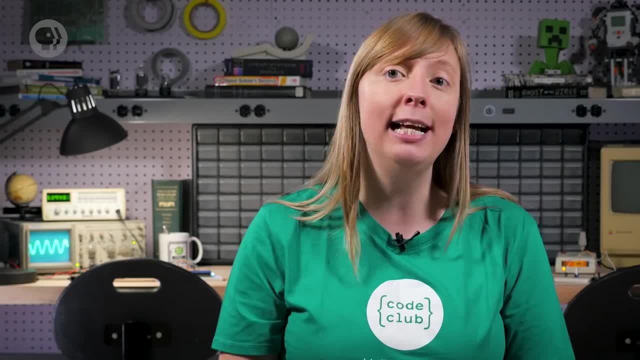 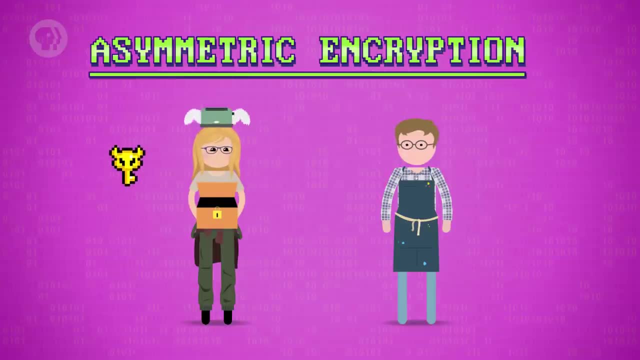 key can decrypt. In other words, knowing the public key only lets you encrypt but not decrypt. It's asymmetric. So think about boxes with padlocks that you can open with a key To receive a secure message. I can give a sender a box and a padlock. 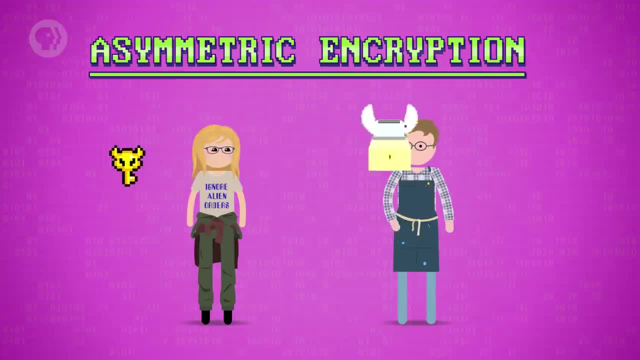 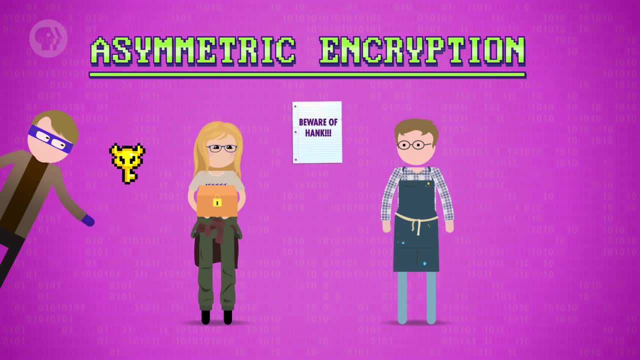 They put their message in it and lock it shut. Now they can send that box back to me and only I can open it with my private key. After locking the box, neither the sender nor anyone else who finds the box can open. 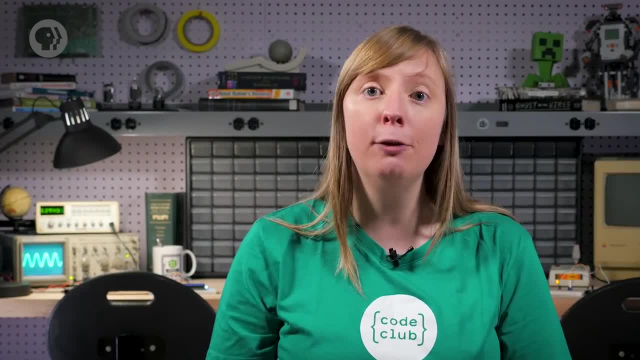 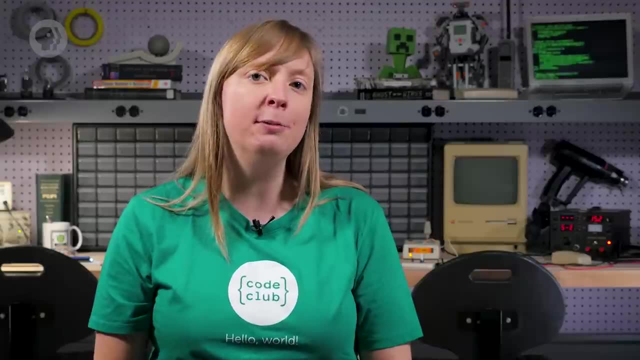 it without brute force. In the same way, a digital public key can encrypt something that can only be decrypted with a private key. The reverse is possible too: encrypting something with a private key that can be decrypted with a public key. This is used for signing, where a server encrypts data using their private key. 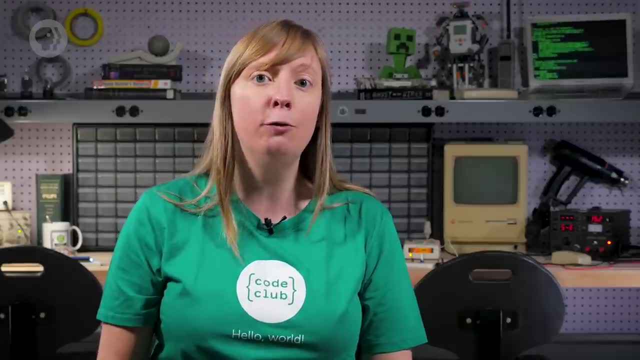 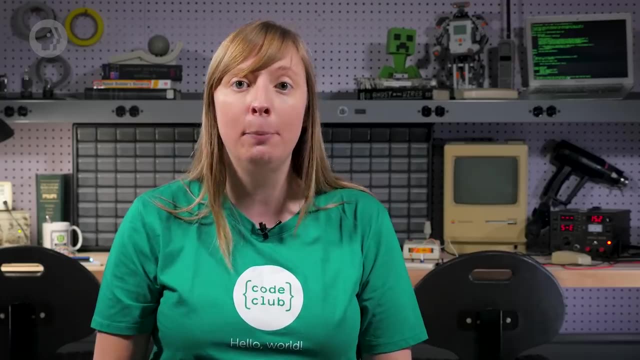 Anyone can decrypt it using the server's public key. This acts like an unforgeable signature, As only the owner, using their private key, can encrypt it. It proves that you're getting data from the right server or person and not an imposter. 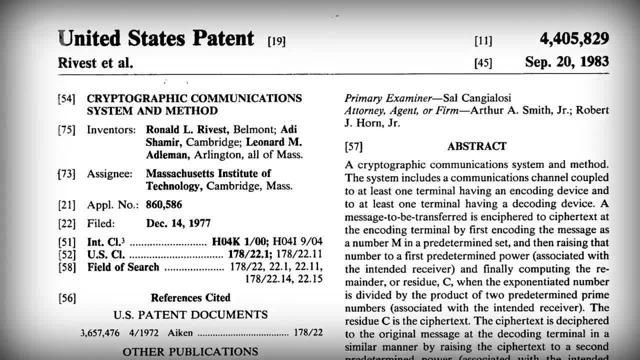 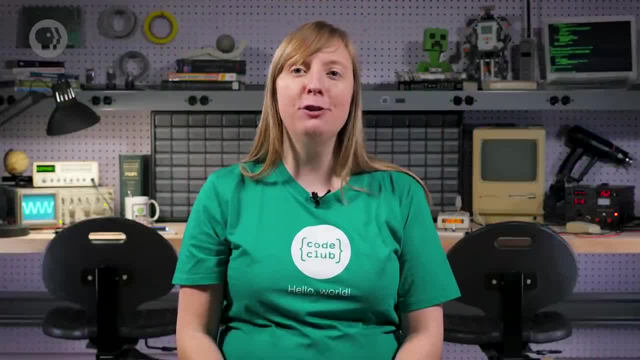 The most popular asymmetric encryption technique used today is RSA, named after its inventors, Rivest, Shamir and Edelman. So now you know all the key parts of modern cryptography: Symmetric encryption, key exchange and public key cryptography. When you connect to a secure website like your bank, that little padlock icon means. 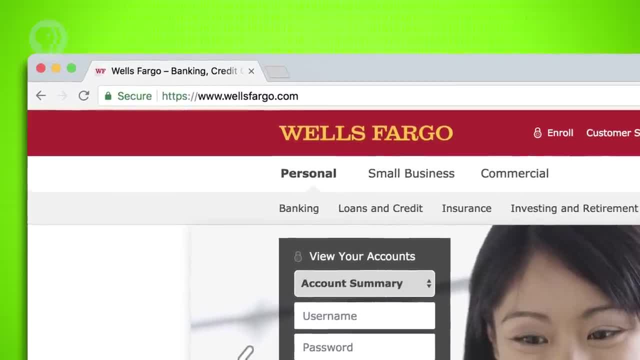 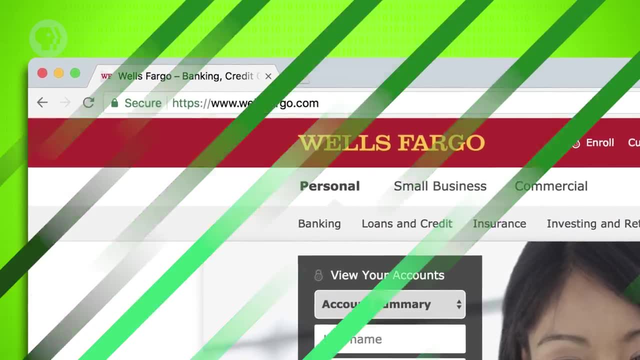 that your computer has used public key cryptography to verify the server. This allows you to establish a secret temporary key and symmetric encryption to protect all the back-and-forth communication from prying eyes, Whether you're buying something online, sending emails to BFFs or just browsing cat videos. 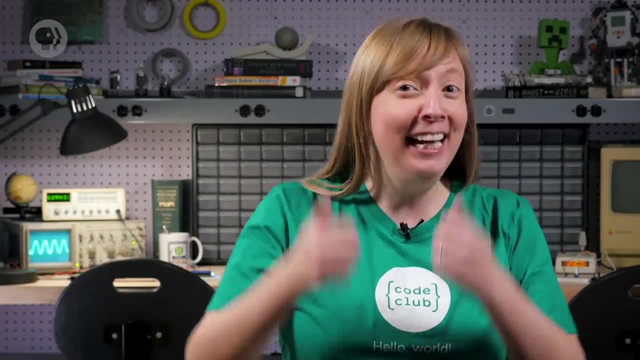 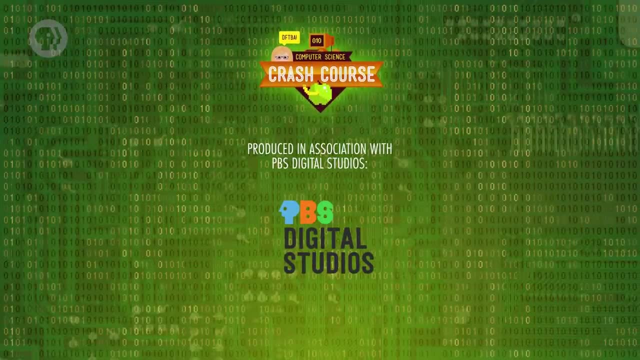 cryptography keeps all that safe, private and secure. Thanks, cryptography. Crash Course Computer Science is produced in association with PBS Digital Studios. At their channel, you can check out our playlist of shows like Eon's Physics Girl and It's OK To Be Smart. 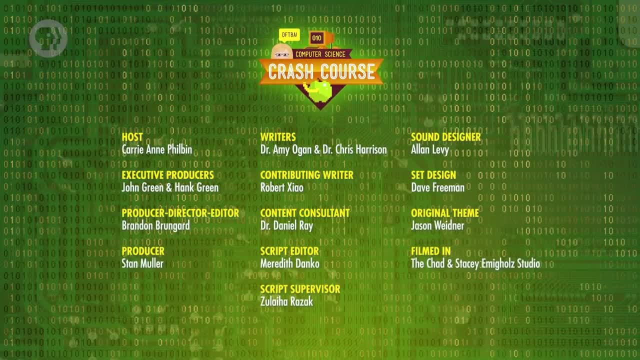 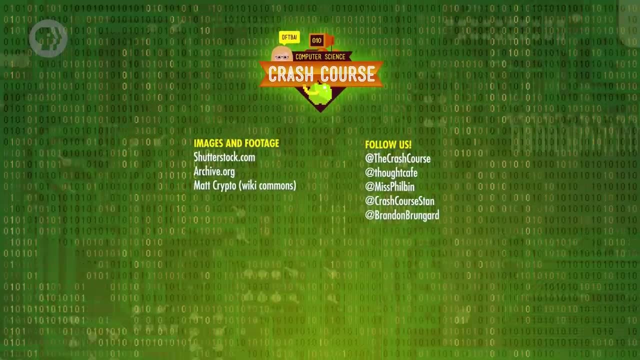 This episode was filmed at the Chad and Stacey Emmergoltz Studio in Indianapolis and it was made with the help of all these nice people and our wonderful graphics team, Thought Cafe. Thanks for the random access memories. I'll see you next time.